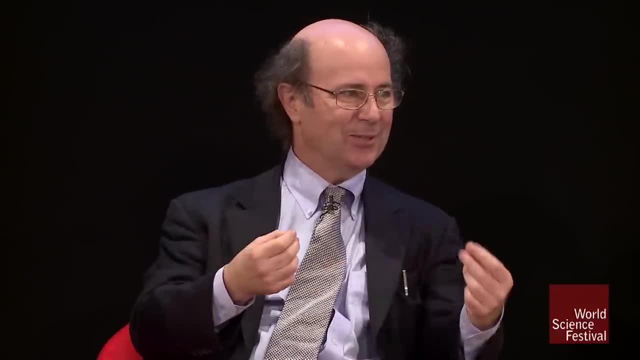 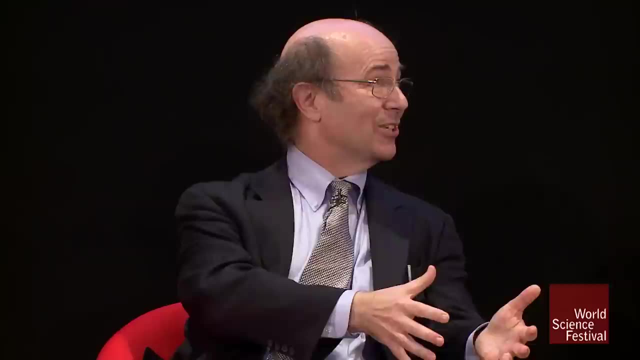 say, changing electrons into quarks and quarks into electrons, And you get different equations, of course, but they have exactly the same consequences as the equations you had before, I see. So no matter how you arrange it, it all adds up. 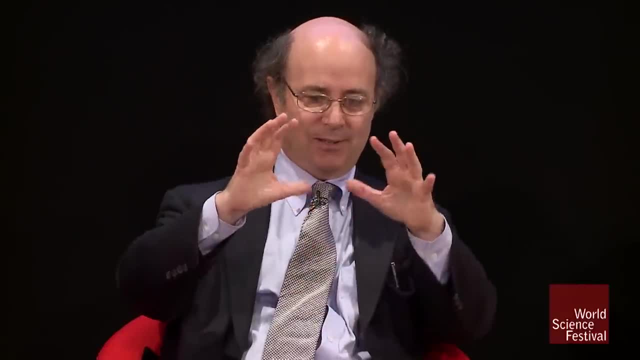 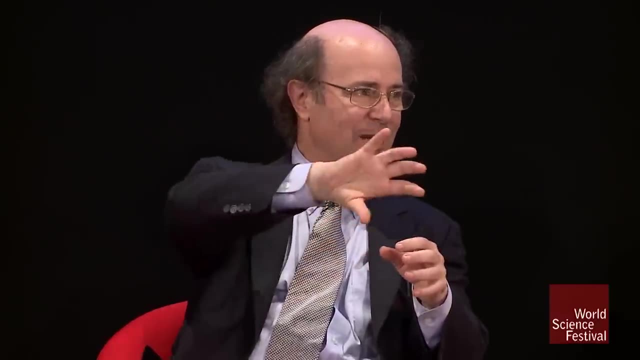 It all looks the same overall. So the idea is similar to the way we say a circle or a sphere is symmetrical because you can rotate it And although every point is in a new place, it's still the same overall shape. 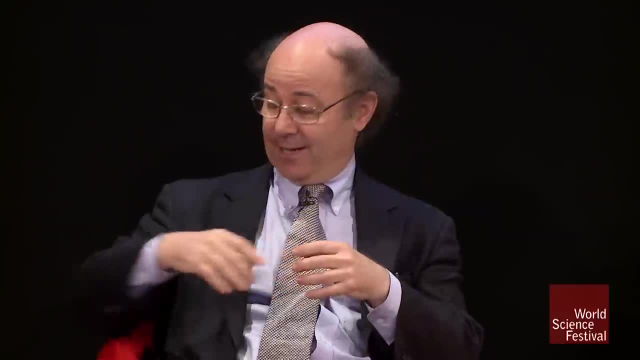 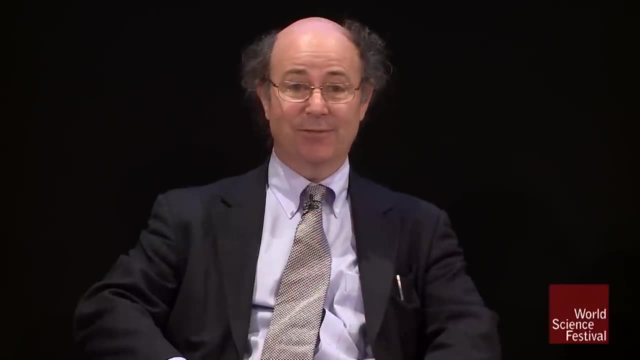 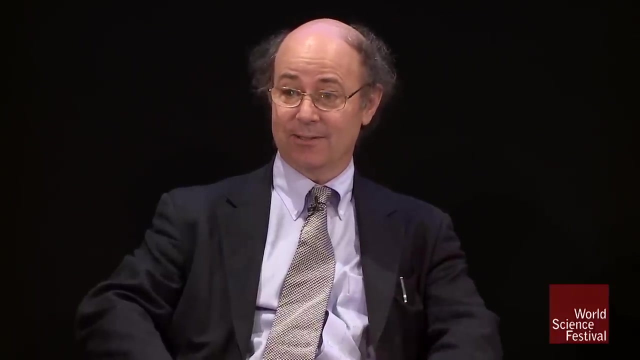 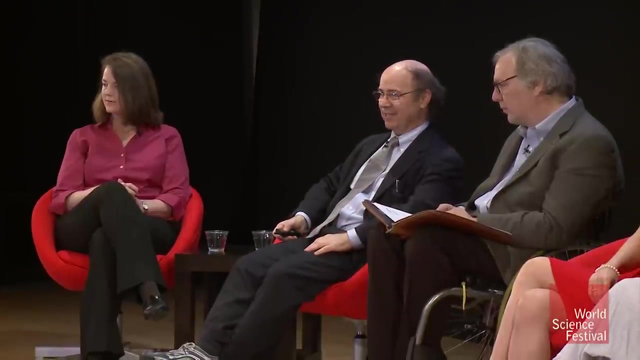 So it's the same idea, but applied to equations. So these are called unified theories that put together electrons and quarks and photons and gluons, and we can write down very elegant theories of this kind. Now next slide, However: a crucial prediction of this kind of idea. if the forces are really going to be all the same, is that they have to have the same strength. At least after you peel away the complications of things like the Higgs field and look down at very short distances and high energies, the different forces should have the same strength. 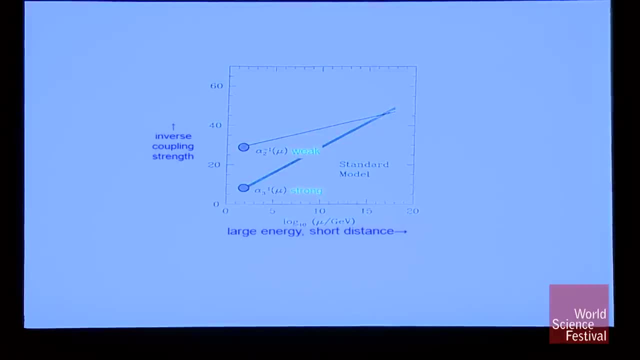 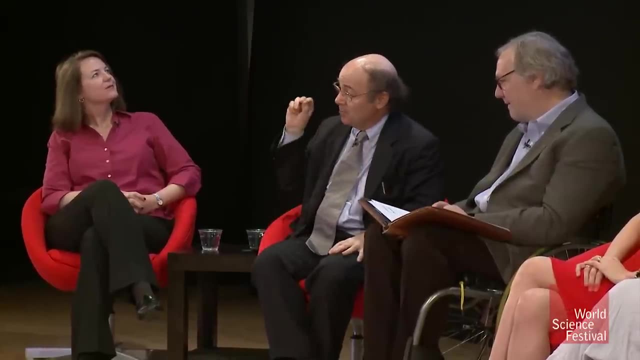 And that refers to the two forces, the weak force, This is weak and strong And strong force. And you can see, on this plot, we make these corrections, peeling away the effect of the Higgs field and we see whether the basic underlying forces, 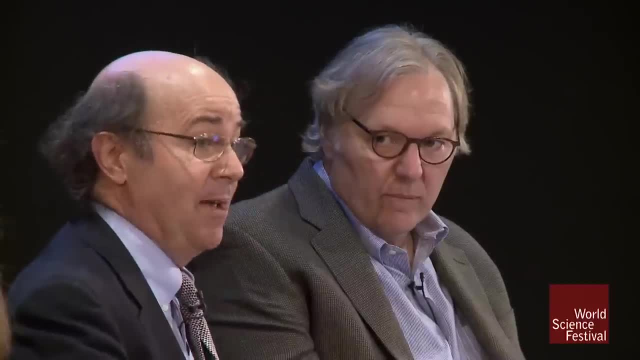 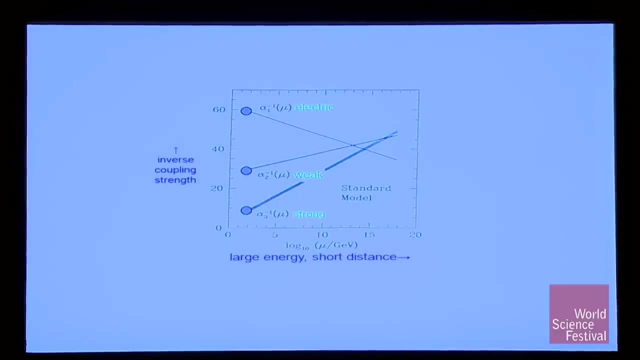 at the shortest distances and highest energies are the same force and have the same strength. We see that if we take the strong and weak interactions and make those corrections to the strength, the lines do indeed cross. So that's encouraging. But on the other hand you might say that two straight lines. 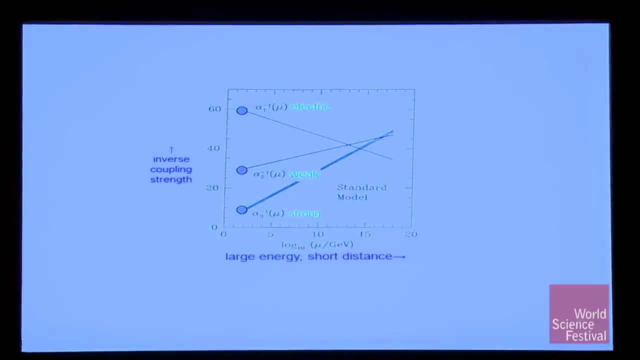 do tend to meet at a point, so it's not as impressive as it could be. But then we have a third force. We can make the correction, We can also compare that and you see, don't almost but not quite. 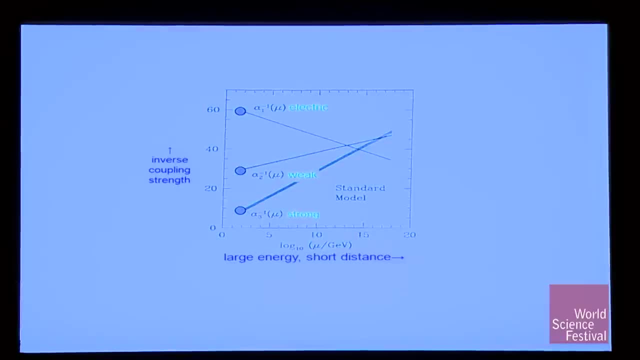 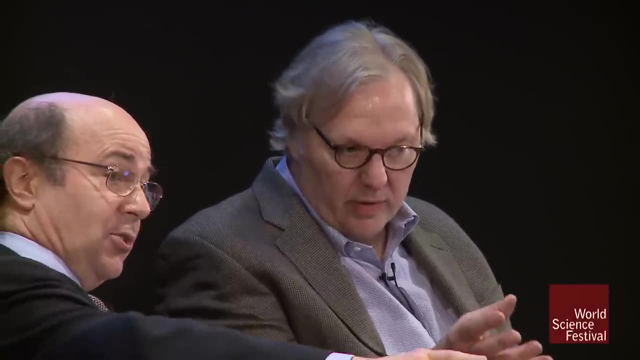 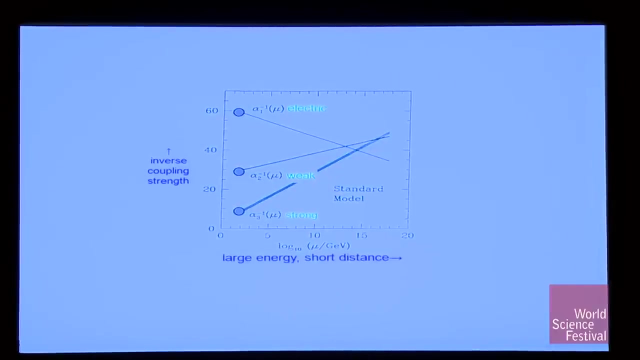 They don't quite all unify Now. so, And this information right here, these graphs, are based on experiments we've already done. Yeah, the little circles on the left are the measurements of the strength that we know about, And then, by the kind of work that I got the Nobel Prize for, 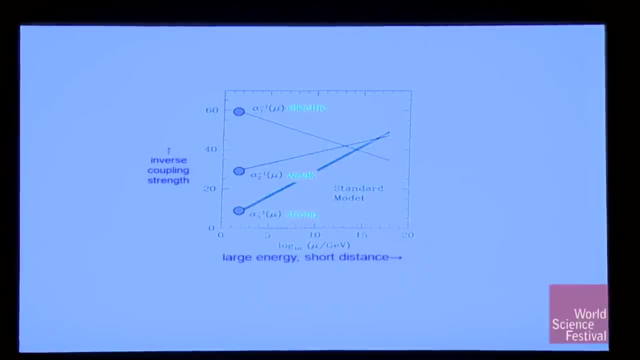 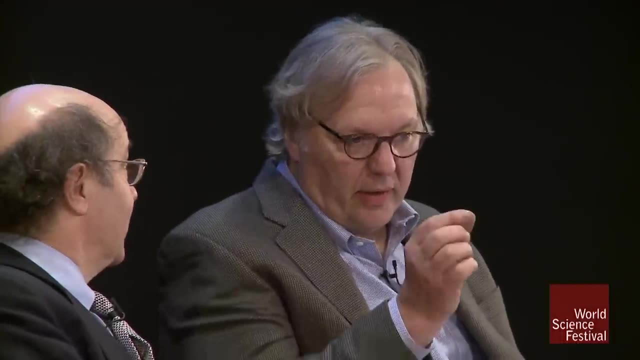 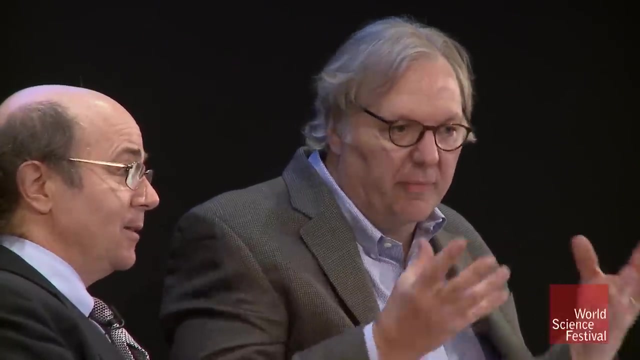 you can calculate how they change as you strip away the complications and go down to shorter distances, And the idea is again that they unify at some energy level and that all of these forces- electric, weak and strong, Right- should come together. 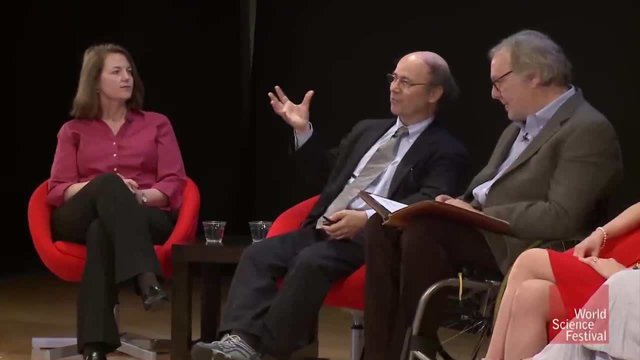 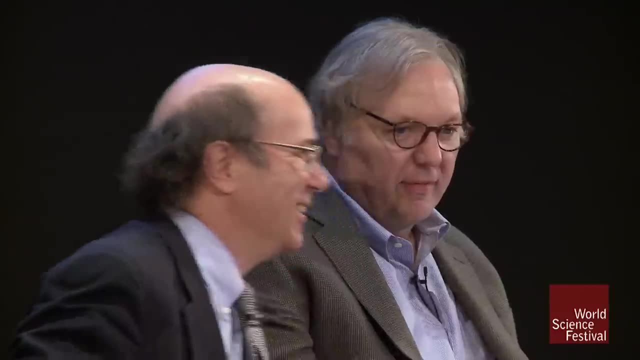 are essentially part of the same stuff. Right, There's one underlying Ur-force that sees them all the same. Would you call it Ur-force? I would. You could come up with a better name than that. People. sometimes It's the same concept as the unified field theory. 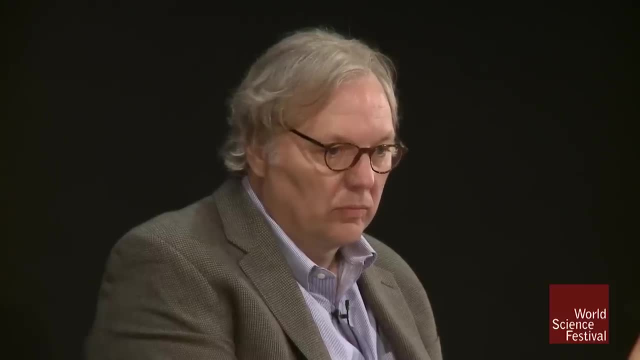 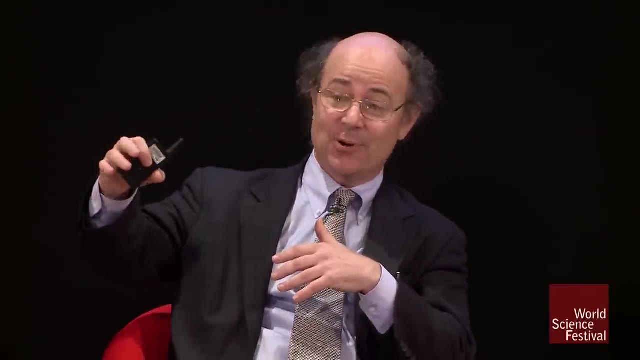 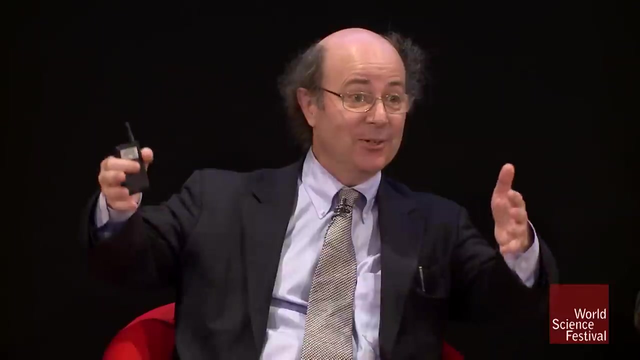 that people have been dreaming about for a long time. So even with the unification I talked about, there were still two different kinds of things. There's electrons and quarks on the one hand, and photons and gluons on the other. So the remaining step is to unify those two things. 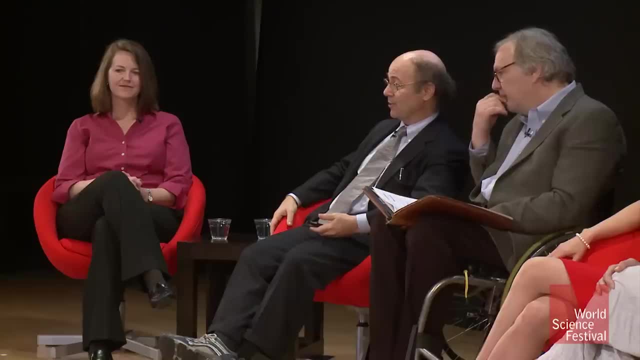 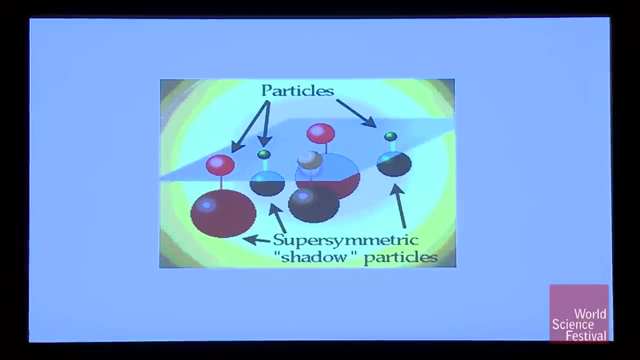 And this is possible using an idea called supersymmetry. According to supersymmetry, there's an extra dimension of space which is not, however, a dimension you could move around in or fly spaceships through or anything like that. It's what's called a quantum dimension. 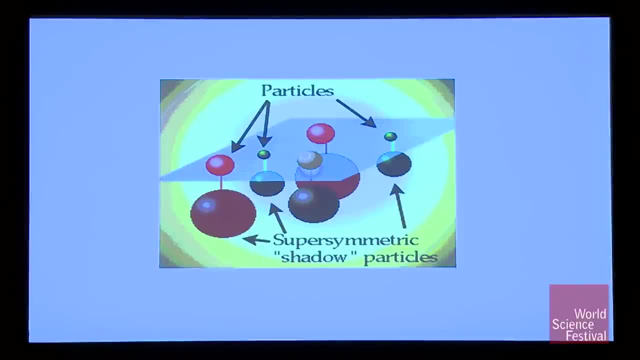 What happens if you move in that dimension is that you change into a very different kind of particle, which would be very uncomfortable, actually, But you would change into a particle that has a different character. So an electron could change into a photon-like particle. 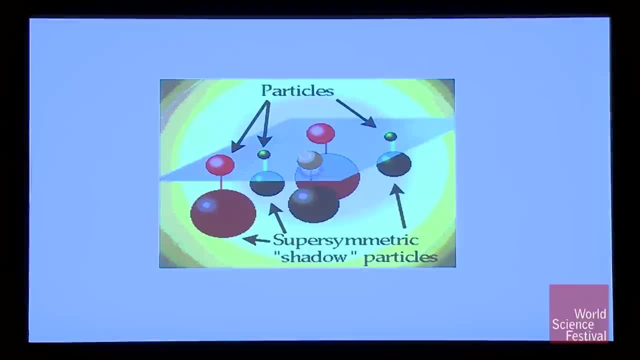 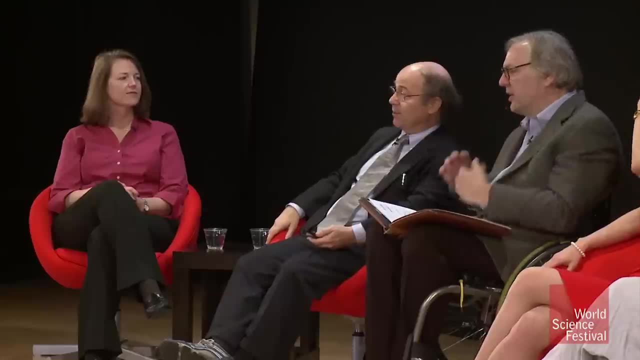 or a quark could change into a gluon-like particle. Is it that it changes or that there is a pair of particles that are kind of channeling each other? It changes. No, it changes, It literally changes. It literally changes. So the mass changes. 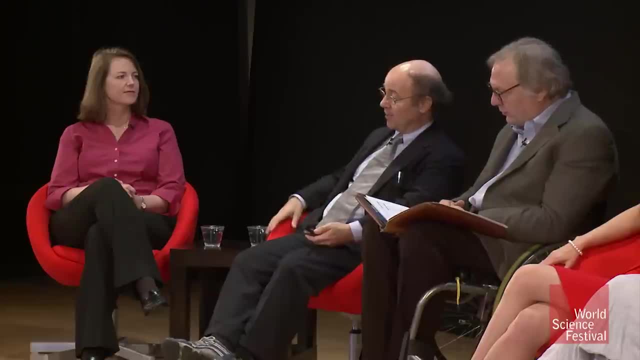 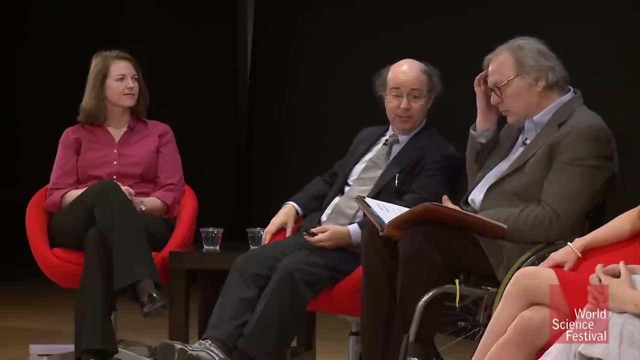 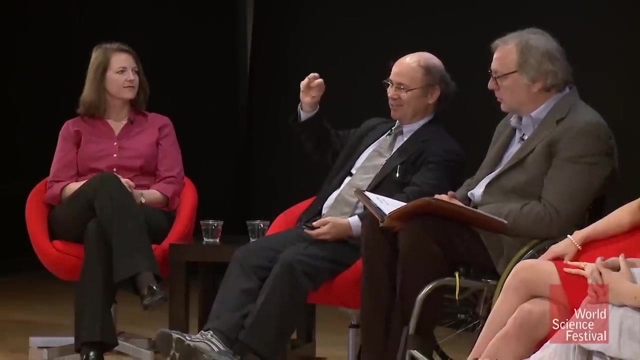 A few properties stay the same, so we can tell that they're related, but the mass changes and the spin changes. So to implement, And that would complete the unification, But to do that we have to introduce new particles. When we introduce new particles, 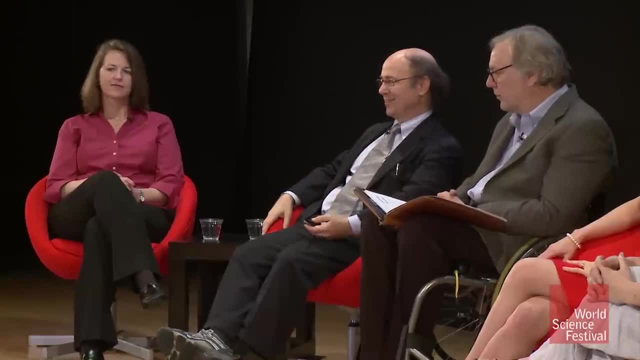 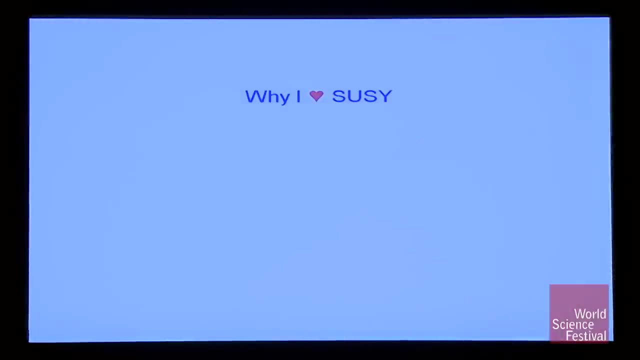 we have different complications to strip away, so we have to redo that calculation. I showed you, Susie is supersymmetry. Keep going, And you see if you do it with supersymmetry. Ah, look at that, now it really comes together.